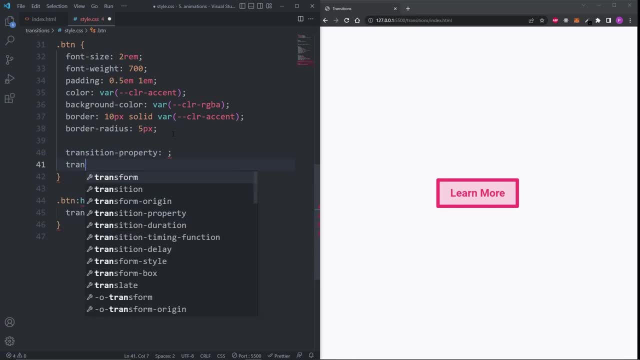 properties: Transition property, transition duration, transition timing function and transition delay. The transition property defines which property the transition effect should be applied to. In our hover state we are only using the transform property, so in here we can say transform. The transition duration defines how long the transition effect should take to complete. 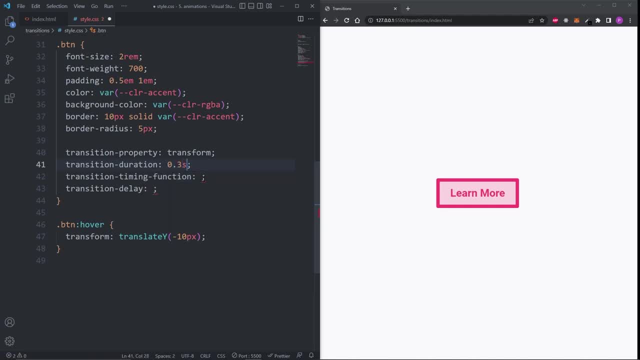 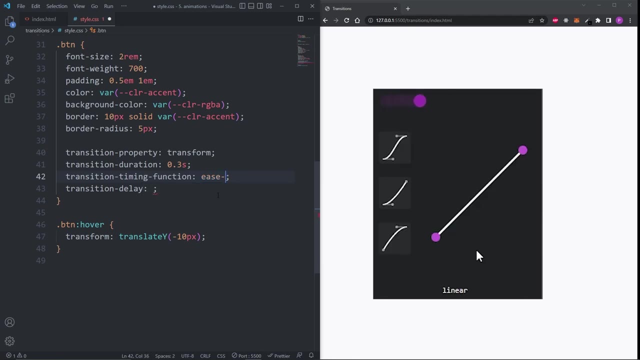 I'm going to set it to 0.3 seconds. The transition timing function defines the acceleration curve for the transition. The common possible values that go in here are: ease in, ease out, ease in out, linear and ease, which is the default. 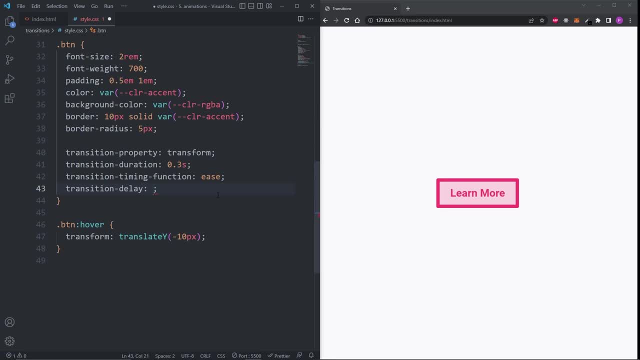 The transition delay defines the delay before the transition should take effect. I want my transition to start the moment the element is hovered on, so I set this one to 0 seconds. When we hover over our button, we see the button moves 10 pixels up over time and this is a lot better than before. but in our code 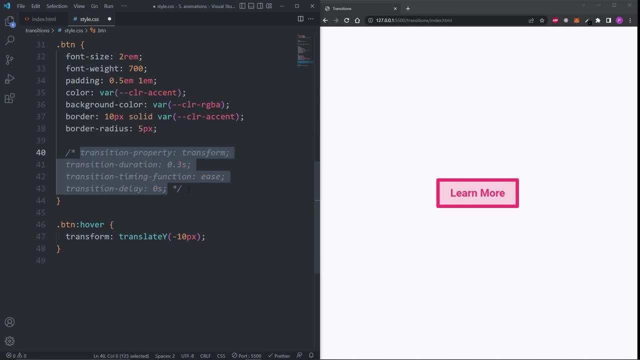 what we can do is, instead of using these four properties, we can use the shorthand property, transition sixth policy. In the transition property, we can set the same values that we passed in the four properties and also in the same order. So transform: 0.3 seconds. 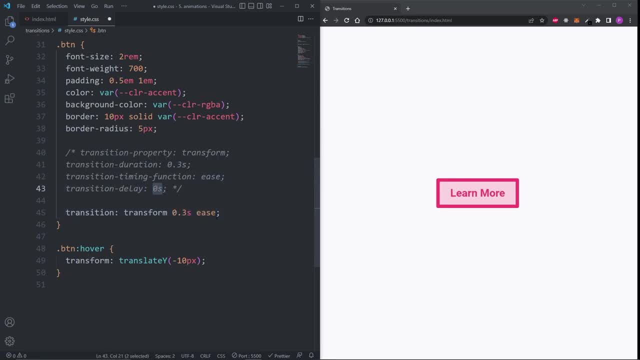 ease: 0 seconds delay. Lower System: 0.4. darkest: 0.8. Perfect, We see this works great. but we can shorten our code even more. If we have a delay of 0 seconds, then we can remove it entirely. So ease sees the default timing function, so we can remove it as well. and now, when we hover over our 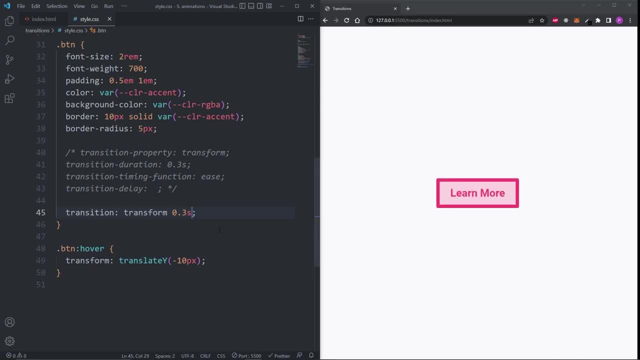 button. we see it's still working perfectly. Sometimes you might have more than one property changing. for example, maybe on hover I want the background color to match the border color and also maybe I want the color of the text to be white When I hover over my button. the only 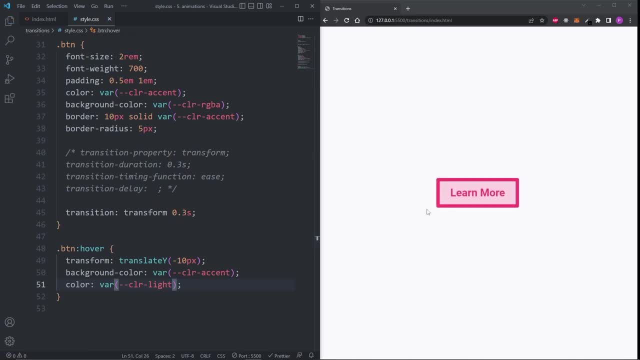 property that has a transition effect is the transform. So what I can do is inside my transition property I can comma separate the different properties. I want animated: The background color property with a 0.3 second duration and the color property with a 0.3 second duration as well. 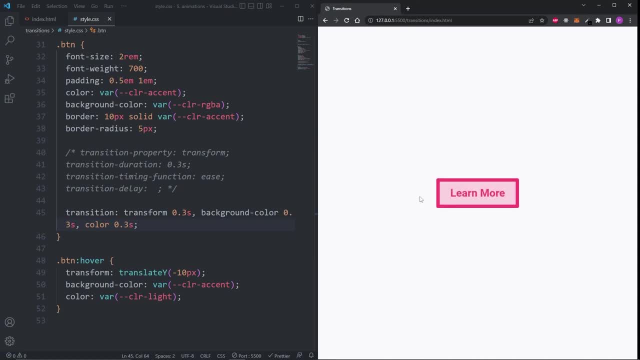 Now, when I hover over my button, everything is being animated. but back in our code, if I had more than three properties on our hover state comma, separating each property would take a lot of time, especially if they shared the same duration, timing function and delay In those cases what we can do. 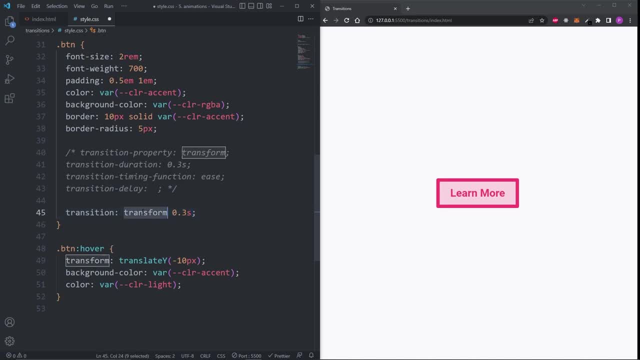 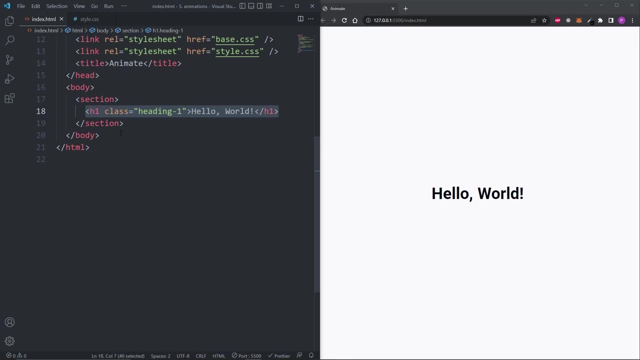 instead is have nothing being comma separated and on the first value, instead of defining a property, we can replace it with the same property. Now everything is going to have a transition effect applied to it. To create an animation, we first need an element that we want to animate. 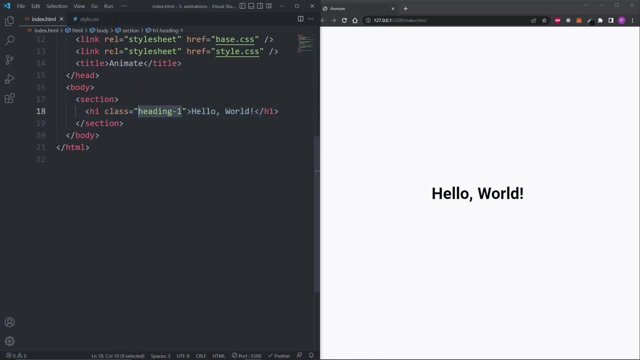 In my html I have an h1 element with the class of heading 1.. To animate this heading I can head over to my css file and add a keyframe. The syntax for this is: at keyframes and curly braces. In between the at keyframes and curly braces goes the name of our animation. I'm going to. 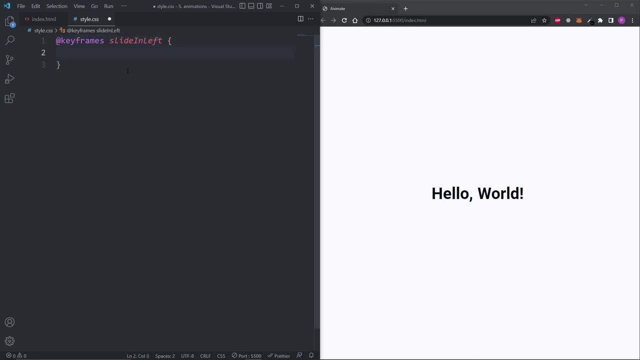 call it slide in left. Inside the curly braces goes the animation. I want my heading to be positioned on the left side of the screen and then slide into its original position. To do this, I need to define the rules from the beginning of the animation to the end of the 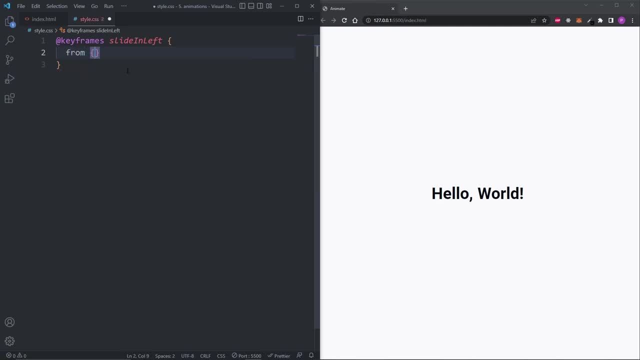 animation. Inside the curly braces I can add the values from and to. From represents the beginning of the animation, or zero percent completed, and the to represents the end of the animation, or 100% completed. They both have curly braces. I want the animation to start 300 pixels to the left. 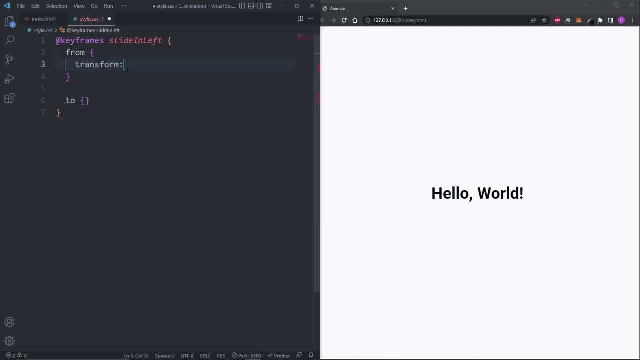 So inside the from curly braces I can add a transform of translate x minus 300 pixels. Then inside the to curly braces I can add a transform of translate x and set it to zero. I set this one to zero because a translate x of zero will bring the element back to its 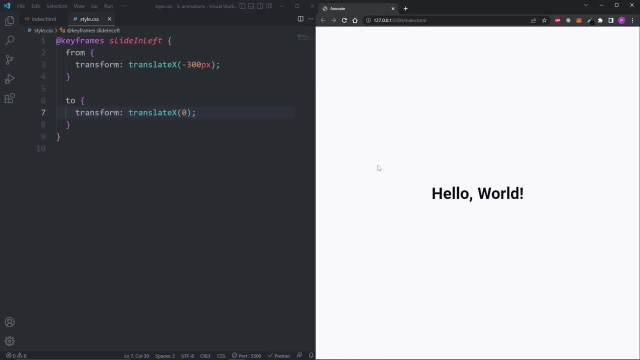 original position. Looking at our heading, we see nothing is happening. This is because we didn't tell our heading to animate. I can select our heading by its class name and in here go seven animation properties: Animation name, animation duration, animation timing function, animation delay, animation iteration count. 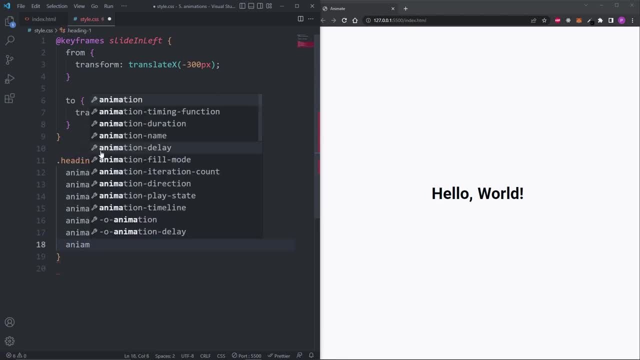 animation direction and animation fill mode. The animation name property is for selecting the keyframe you want to use to animate the element. We created a keyframe called slide in left, so in the animation name property as a value I will pass it slide in left After setting the animation name. 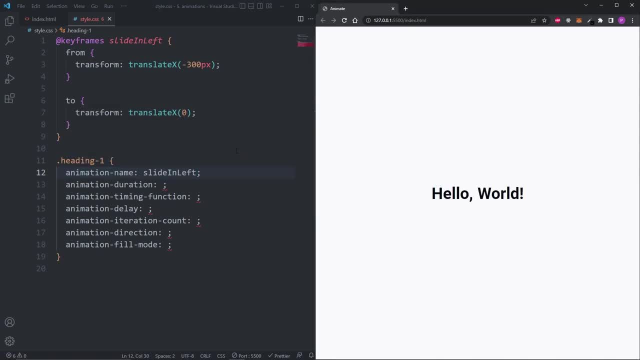 property. we see our heading is still not animating. This is because we need to set the animation duration. The animation duration property sets the time it takes for the animation to complete one lap. When you create a keyframe animation, you're defining the rules of the animation for. 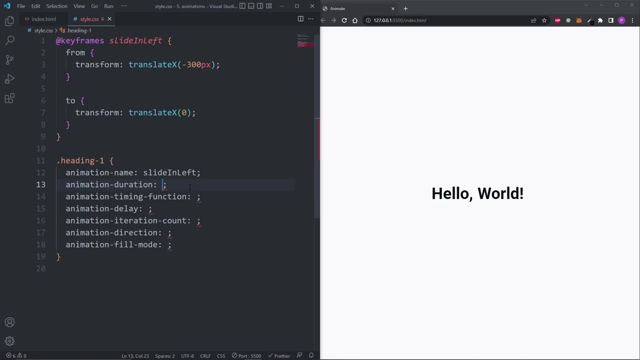 0% to 100%. This property defines how long it takes to animate from 0% to 100%. The default is 0 seconds, but if I leave it at 0 seconds, our animation will never run, so I'll set it to 1. 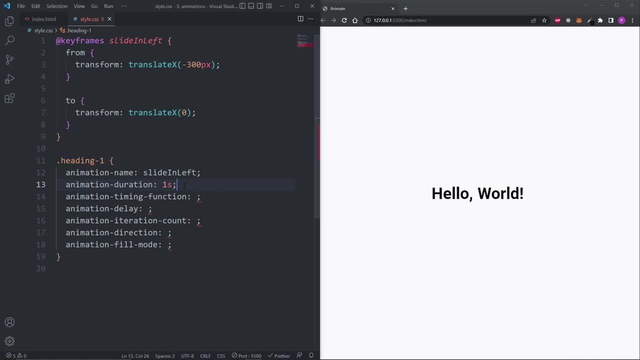 second. Now we see our heading is being animated. The animation timing function property defines the acceleration curve for the animation. The default is ease, but we have the same options as before: Ease, ease in, ease out, ease in out and linear. I'll set mine to ease in. 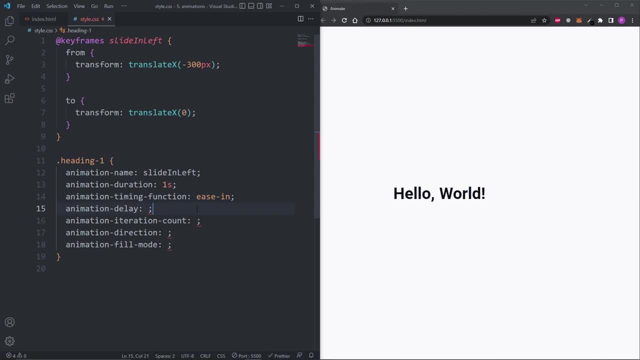 The animation delay property sets a delay before running the animation. The default is 0 seconds and this means the animation will run right away on page load. I will leave it at the default 0 seconds for now. The animation iteration count property defines how many times you 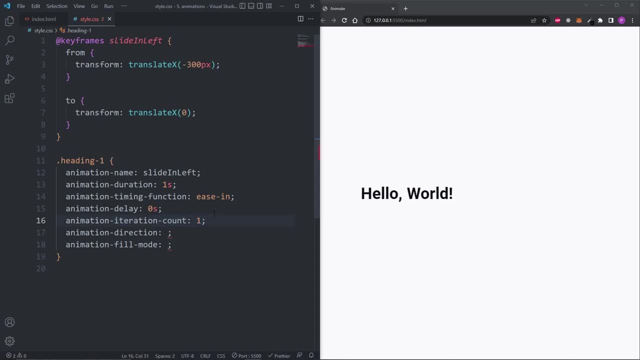 want the animation to run. The default is 1, and this means the animation will complete one lap and then stop animating. If I set it to 2 or more, then the animation will run 2 or more times. I can also set it to infinite. 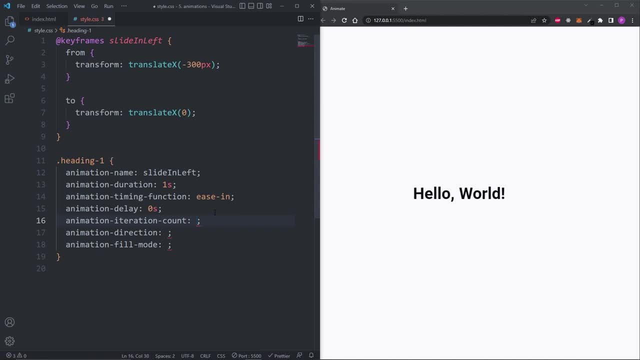 and this will make the animation run forever. I will leave it at the default value of 1.. The animation direction property defines whether the animation will run normally or in reverse. The default is normal, but if I set it to reverse, all this will do. 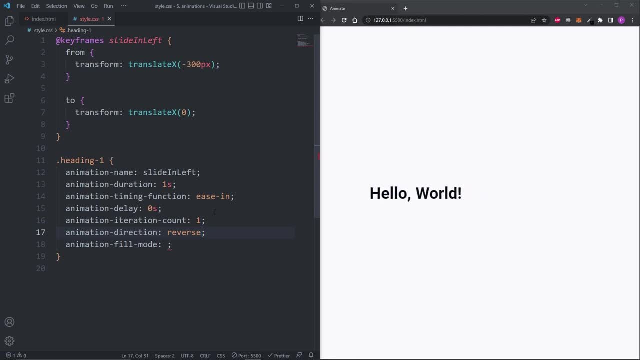 is start the animation from the last keyframe and end it on the first keyframe. I will leave it at the default value of normal. The animation fill mode property defines how the animation will apply the styles from our keyframe before and after its execution. This is hard to understand. 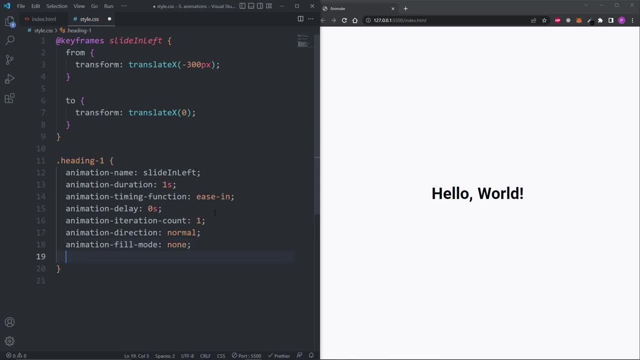 without some visuals, so I'll give it the default value of none. I'll add a transform to our heading of translate Xить minus 150 pixels and I'll add an animation delay of 1 second. The beginning position of our animation is still 200px. 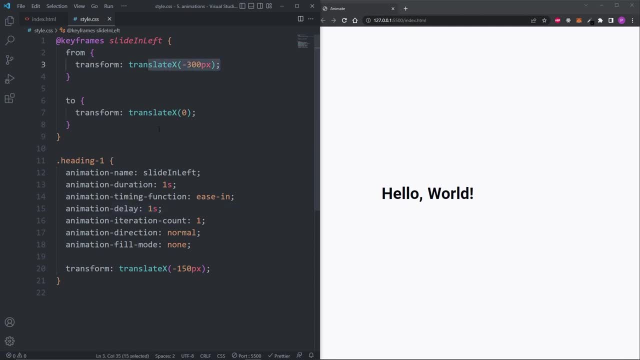 pixels to the left and the ending position of our animation is still in the middle of the page. Our heading, however, now has a transform x of minus 150 pixels. This didn't change the original position of our heading. our original position is still in the middle of the page, However. 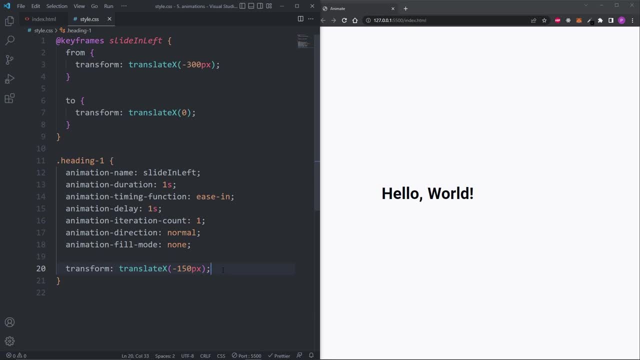 the transform that we added in the heading will push the heading 150 pixels to the left before the animation starts and after the animation ends. We can see this when we look at our heading: It's 150 pixels to the left and after a one second delay the animation starts. 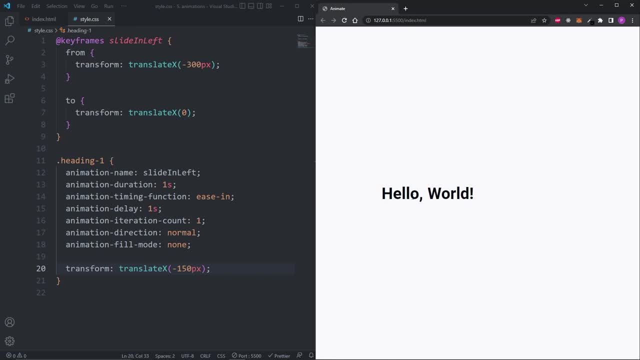 and then, when the animation is over, the heading gets pushed back 150 pixels to the left. We can use the animation fill mode property to change this behavior, If I set it to forwards, although the heading starts 150 pixels to the left when the animation ends, instead of pushing. 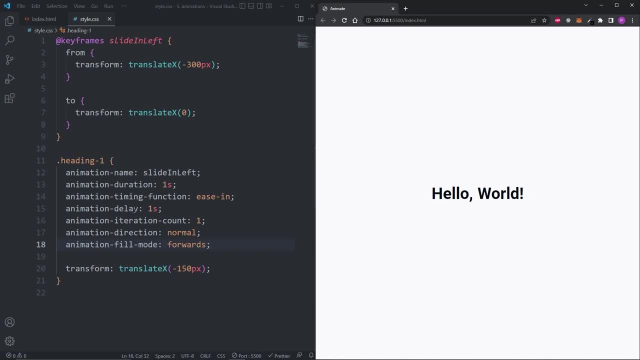 the heading back 150 pixels to the left, like before. we see now the heading stays in the middle and this is because it says forwards will apply the styles from the last keyframe to our heading when the animation ends. If I set it to backwards, the heading will start with the styles that are defined. 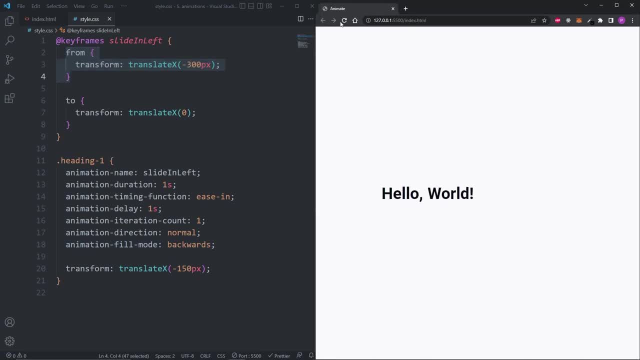 in the first keyframe, but when the animation ends backwards does nothing and the heading gets pushed 150 pixels to the left again. Finally, if I set it to both now, the heading starts with the styles from the first keyframe and ends with the styles from the last keyframe. 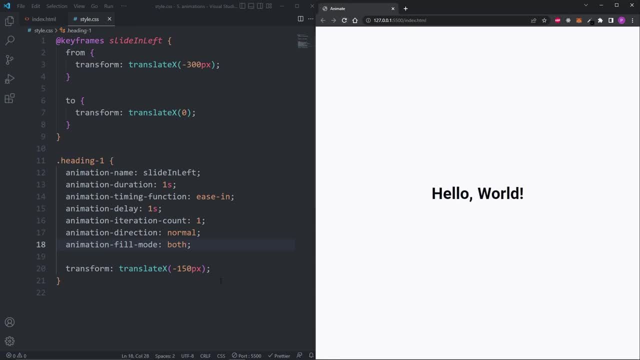 With animation fill mode set to both, the element is never getting pushed 150 pixels to the left because it's saying the element needs to start with the styles from the first keyframe and needs to end with the styles from the last keyframe. This animation property is definitely the hardest one to understand, but hopefully now it makes sense. 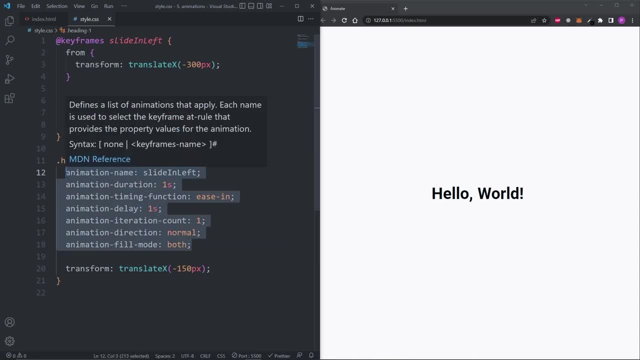 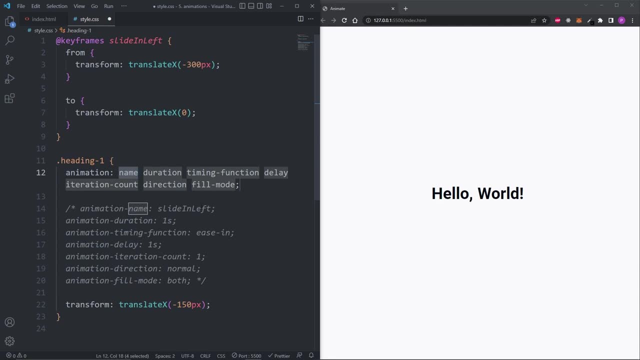 Writing these 7 properties each time you want an element animated is way too much work. We can use the animation shorthand property. It takes the same 7 property values: name, duration, timing function, delay, iteration, count, direction and fill mode. I'll just copy and paste the values. 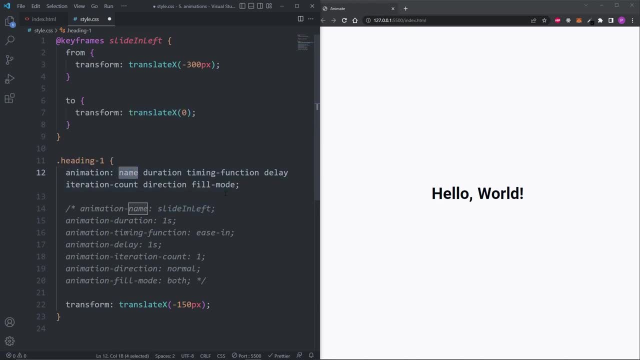 we had in the individual properties into the animation. shorthand. Name is slide in left, duration is 1 second, timing function is ease in, delay is 1 second, iteration count is 1, direction is normal and fill mode is both. I can now delete the individual animation properties and we see: 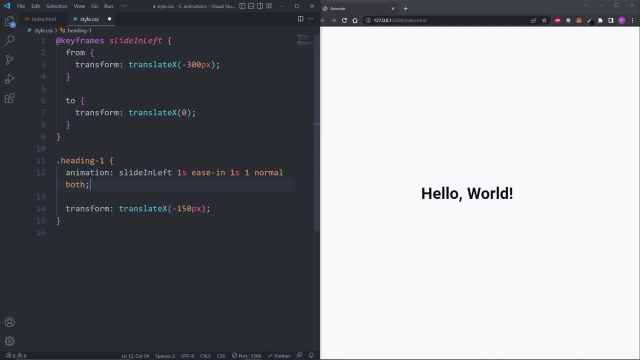 our heading is still animating like before, but now we're only using one property instead of 7.. We can make it even shorter by removing all of the default values. Our iteration count and duration are both set to their default values, so I can just remove them entirely and our animation will still work the same. 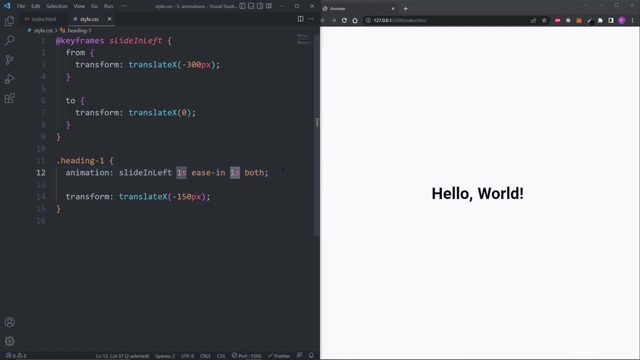 We currently have a delay of 1 second. I'd prefer there be 0 delay, so instead of saying 0 seconds, what I can do is just remove it entirely, because 0 seconds is the default delay value. I can remove the transform that I added earlier, and now that it's gone, I don't really need the 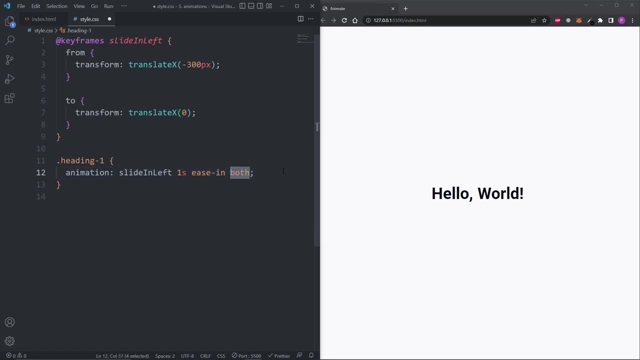 fill mode to be at both. it can be at its default value of none, so I'll just remove it entirely. Our animation is still behaving as we intended, but now look at how clean our code is. Currently, our animation is placed on the element itself. this is bad for reusability. 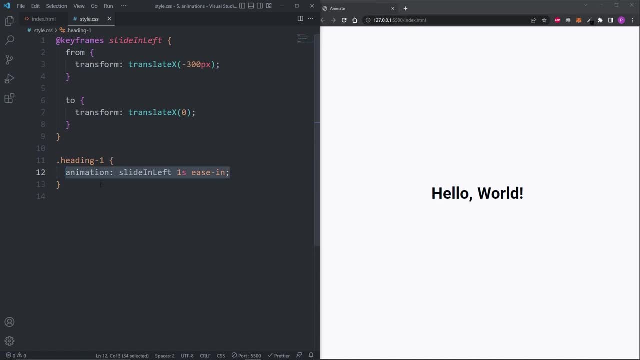 Instead of selecting the heading element by its class name and giving it the animation, what I'll do is create a utility class specifically for the slide in left animation and give it the animation property with all of the same values. Our heading isn't being animated anymore. this is because we need to head over to our HTML. 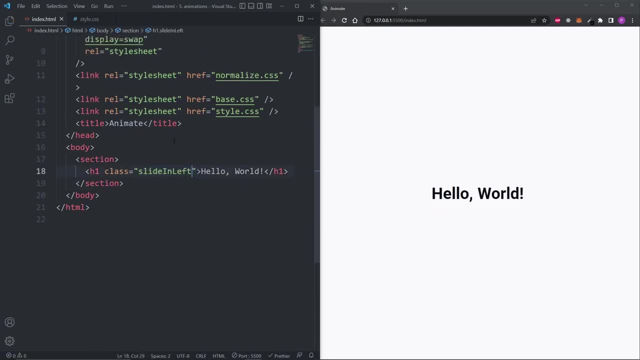 and give our heading the slide in left- utility class. This is superior, because now, if I had other elements that also wanted to have the same animation, instead of selecting them in the CSS and giving them the animation property, all I have to do is give them the utility class and they will animate the same. 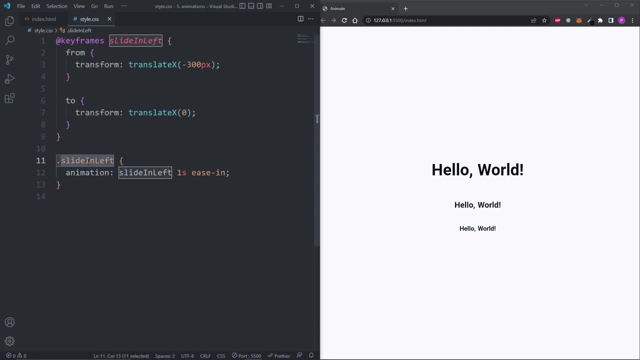 but this way we're saving code by reusing the slide in left utility class. Actually, we can push this utility class architecture even further. At the very top of our CSS file, I'll add a comment saying utility classes. I'll also add a comment right above our keyframe saying animations. 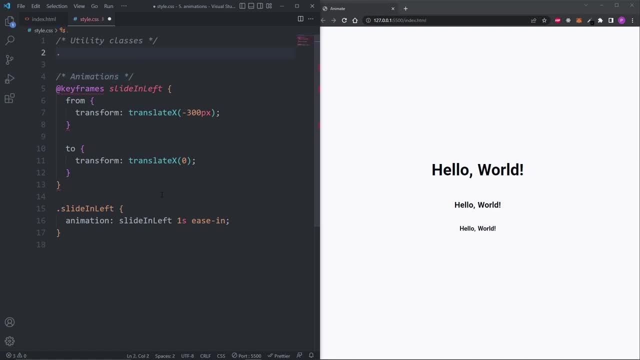 Underneath our first comment. I'm going to have 5 utility classes. the first one will be called animate, with the property of animation duration set to 1 second and the animation fill mode set to both obrajpg. The second utility class is going to be called animate--infinite, with the property of animationIterationCount set to infinite. 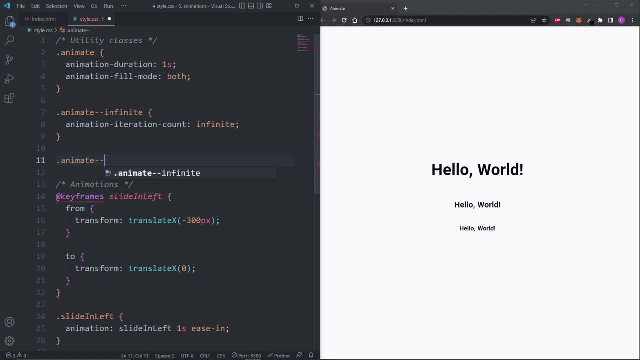 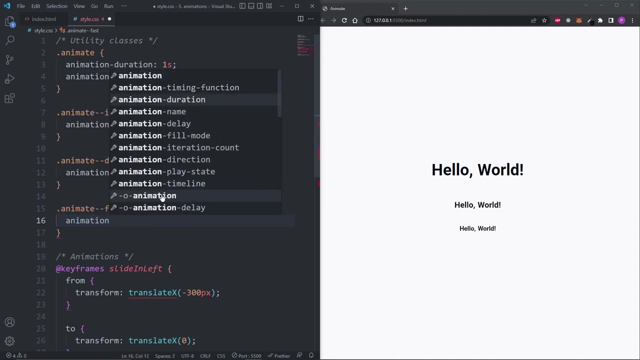 The third utility class is going to be called animate-delay-1second, with the property of animationDelay set to 1 second. The fourth utility class is going to be called animate-fast, with the property of animationDuration set to 0.6 seconds. 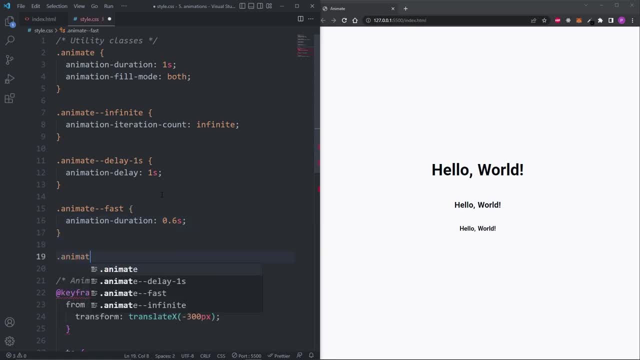 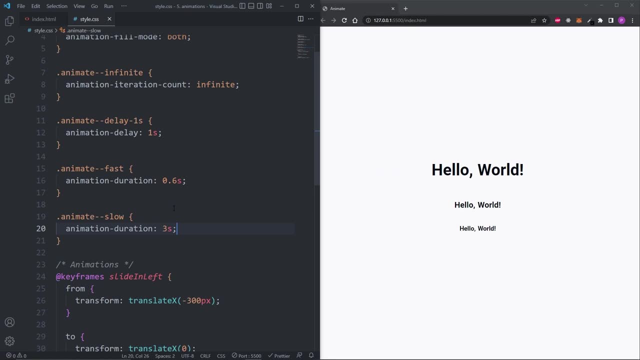 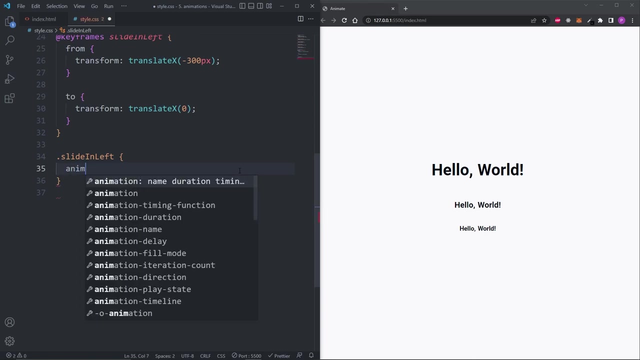 The fifth utility class is going to be called animate-slow, with the property of animationDuration set to 3 seconds. And finally, the last thing we need to do is go to our slide-in left class and replace the animation shorthand with the animationName property set to the name of our keyframe. 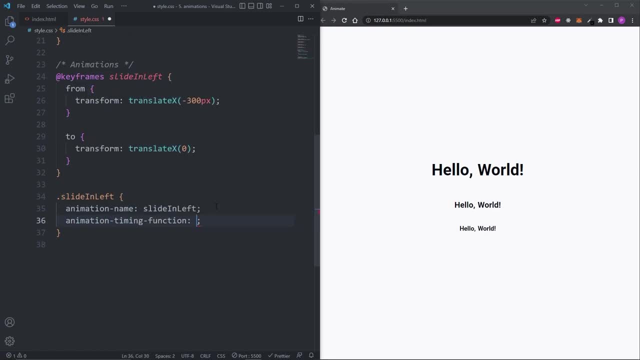 and the animationTimingFunction property set to whatever acceleration curve we want. I'll set it to ease in Now with this architecture. the way it works is over in the HTML. every element I want animated I give the animate class. I want them all to be animated, so I'll give them all the animate class. 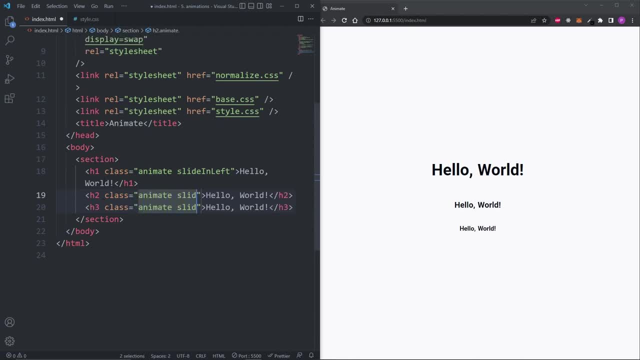 Then I can select the animation I want. In our case we only have one animation, the slide-in left animation. So in the classes of each element I'll give slide-in left. We see, now all our elements are being animated. What we can do now is use the different utility classes where we want. 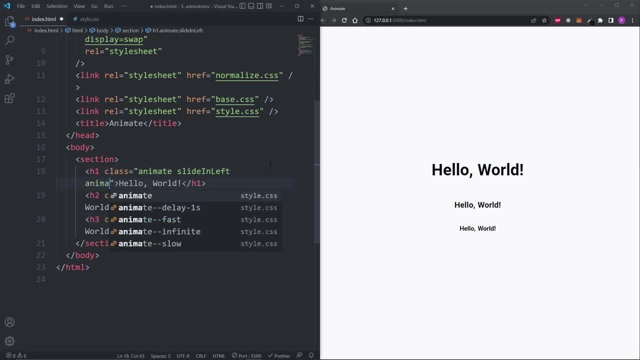 For example, maybe I want the first heading to be fast. I can give it the animate dash dash fast utility class. And now we see our heading is faster than the others. Maybe I want the second heading to be slow. I can give it the animate dash dash slow utility class. 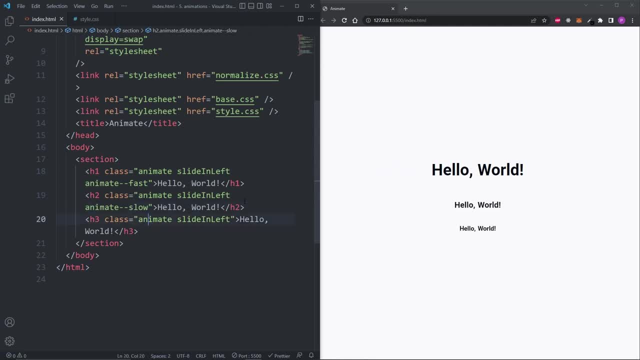 And now it's animating slower than the others. And finally, maybe I want the third heading to have a delay of one second and constantly repeat its animation infinitely, for whatever reason To do this? I can give it the animate dash dash, slow utility class. 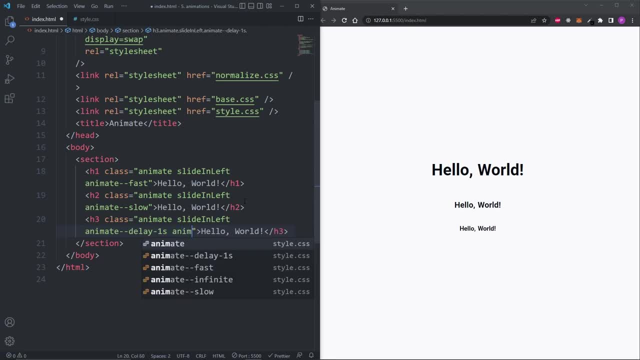 I can give it the animate dash dash delay one seconds utility class And the animate dash dash- infinite utility class. We can make this architecture even better by using double classes In our CSS. I can prepend the animate class to each of these four utility classes. 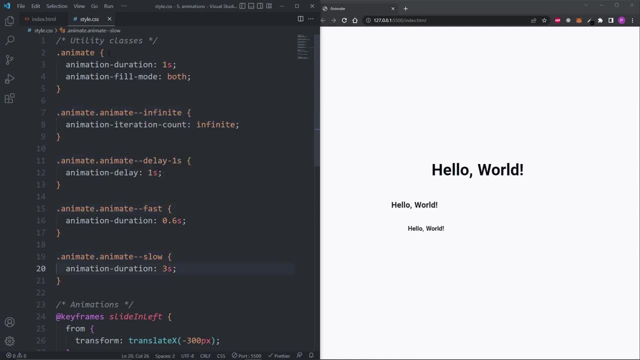 And what this does is it only allows the utility classes to work if the animate class exists in the same element. This can help us avoid any possible accidents that may occur when naming our classes. With this way of working with animations, we can essentially create our very own mini animation library. 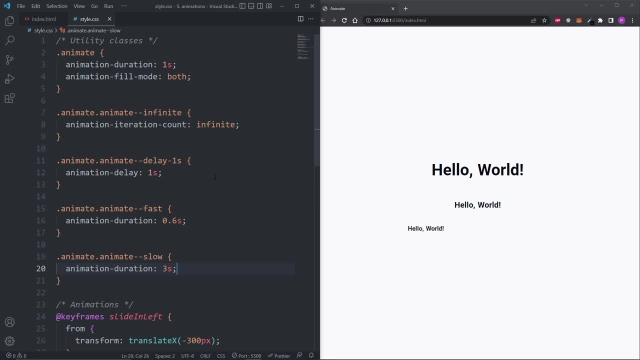 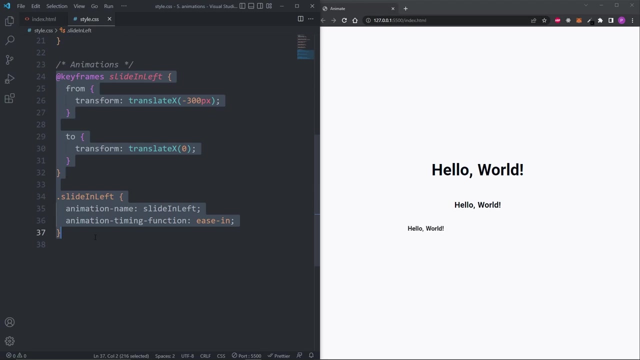 And the reason this works so well is because we decoupled the relationship between the animation and the element, Making each animations a reusable utility class. Well, we only have one animation, so let's add a few more. We can give our slide in left a brother called slide in right. 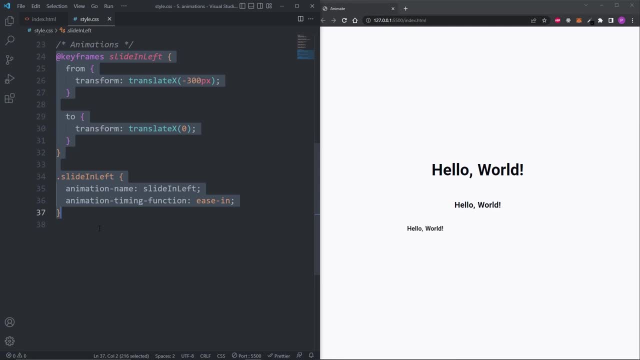 Because this animation will be the same, but come in from the right. I'll just copy the code from our slide in left and paste it underneath. We can rename the keyframe from slide in left to slide in right. We can do the same with the class name and the animation name property. 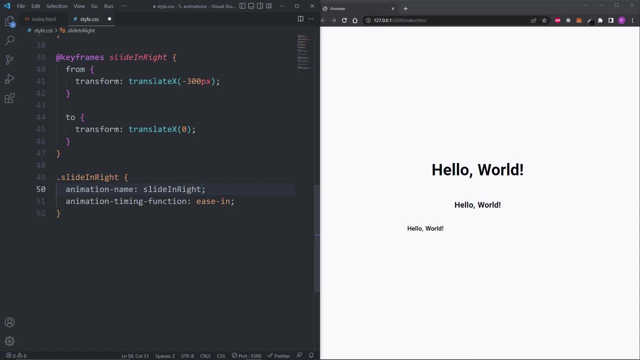 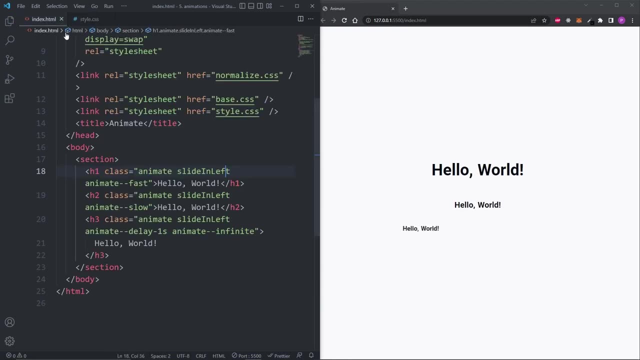 Then in our transform of translate x minus 200, I can just remove the negative and now the element will come in from the right instead In our HTML. I'll give the second heading the class of slide in right instead of slide in left. 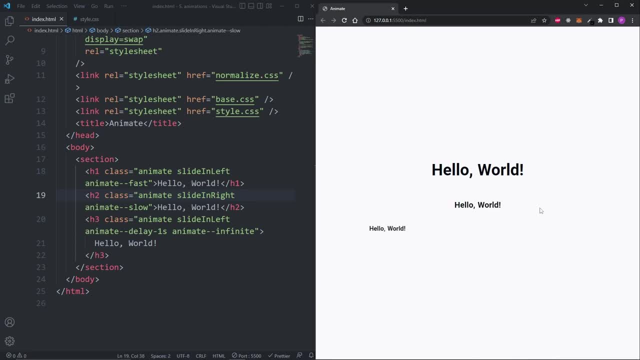 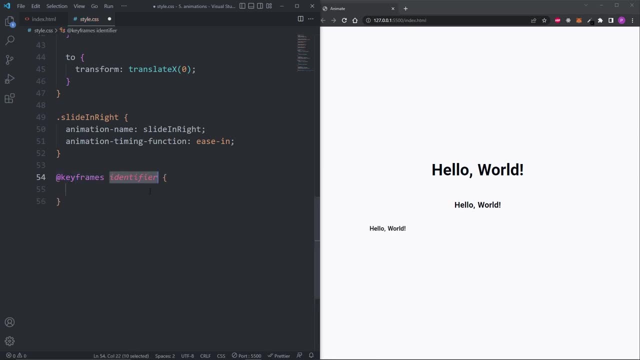 And now we see our heading is coming in from the right. Back in our CSS, at the bottom of the file, I'll add a new keyframe called rotate. It's going to start with a transform of rotate set to 0.. And it's going to end with a transform of rotate set to 360 degrees. 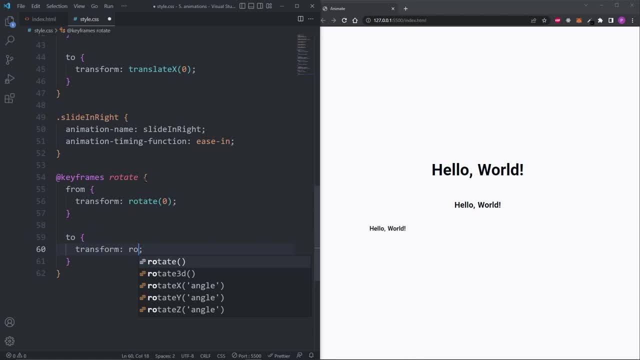 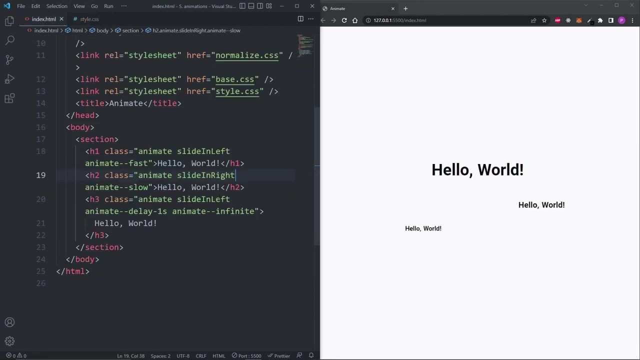 Underneath our keyframe I can add the rotate class and give it the animation name of rotate, And I'll also give it the animation timing function set to linear. Then in our HTML I'll give it the animation name of rotate. In our last heading I'll replace slide in left with rotate. 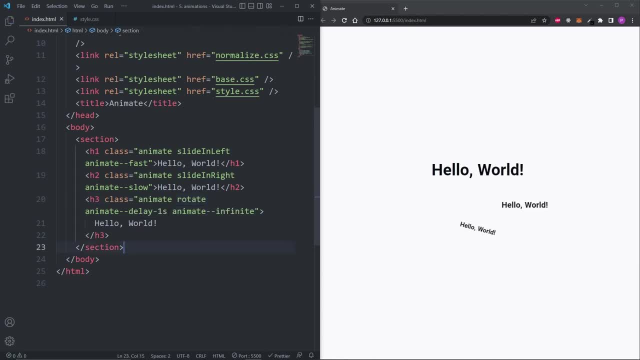 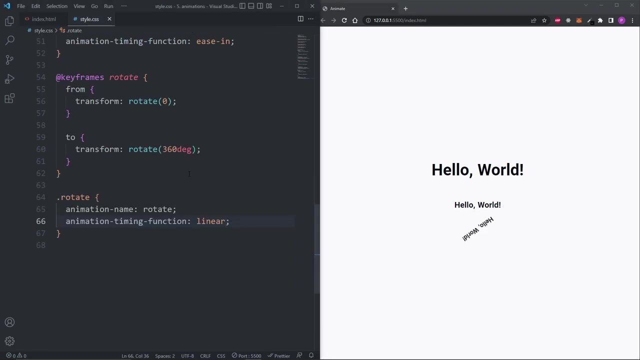 I'll leave the animate dash dash infinite utility class, but I'll replace the animate dash dash delay of one second with animate dash dash slow. And now we see, our last heading is rotating from its center point infinitely. This is what I want, But say, for example, I wanted the heading to rotate, not from its center. 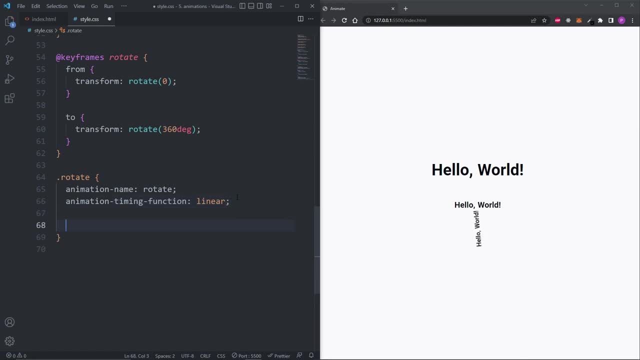 but from one of its corners. What I can do is, in the rotate class, give it the transform origin property, which has a default of center, and set it to top left. Now the last heading is still rotating, not from its center point. 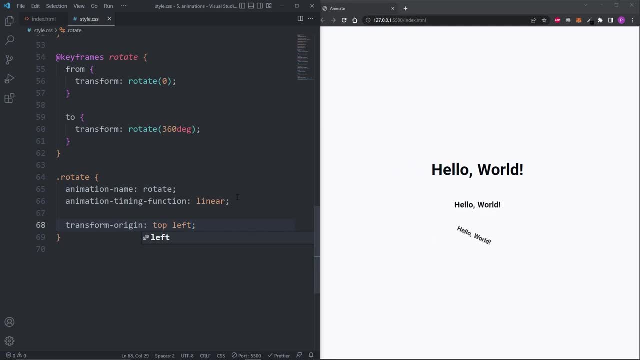 but from its top left corner. I'll do one last animation, this one more challenging than the others. I'll create a new keyframe at the bottom of the file called bounce. I'll also create the bounce class now instead of later, and give it the animation name of bounce. 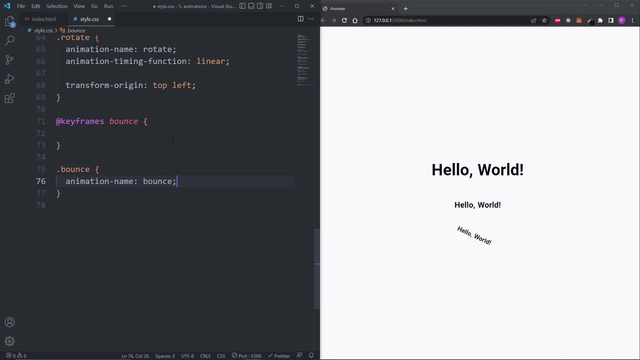 I don't need to give it the animation timing function because I want the acceleration curve to be ease, and ease is the default In my HTML. on the first heading, I'll replace slide in left with bounce and I'll remove the animate dash, dash fast. utility class. 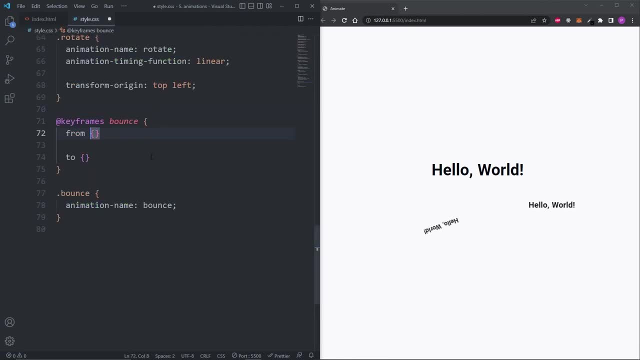 What I want to do with this animation is have the element bounce almost like a bouncing ball. This can be done entirely with the transform of translate y, because our animation will be vertical. The bouncing animation starts on the ground, so I'll set the start of the animation with a transform of translate y of 0.. 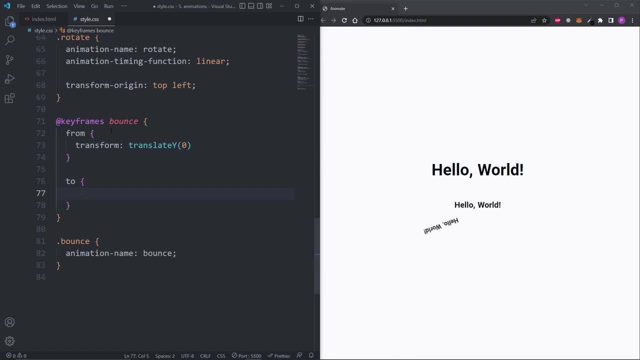 The end of the animation needs to also be on the ground, so I'll set it to 0.. Now what we need is some in-between animations. To do this, we can replace our from and to with 0% and 100%. 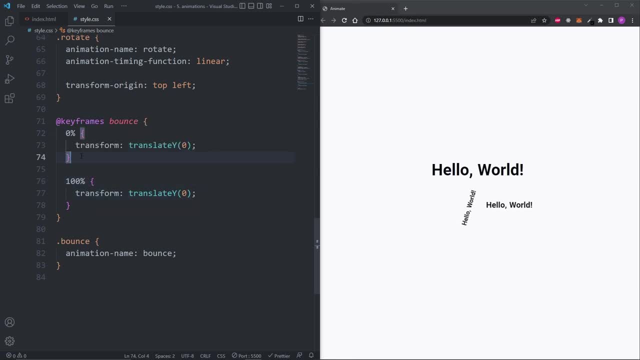 And by using percentages we get more control over the keyframes, because now I can set some in-between values, like 40%, which I'll set here. For example, I can set the value of the fixed value of 0% to a translate y of minus 30 pixels. 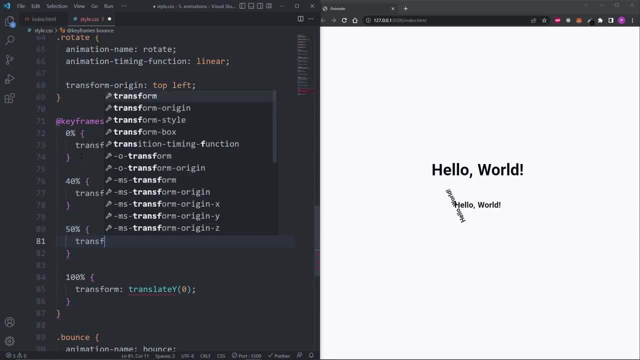 Our heading is going up and down but not really bouncing. I'll add a 50% with a transform of translate y set to 0, and I'll add a 60% with a transform of translate y set to minus 15 pixels. 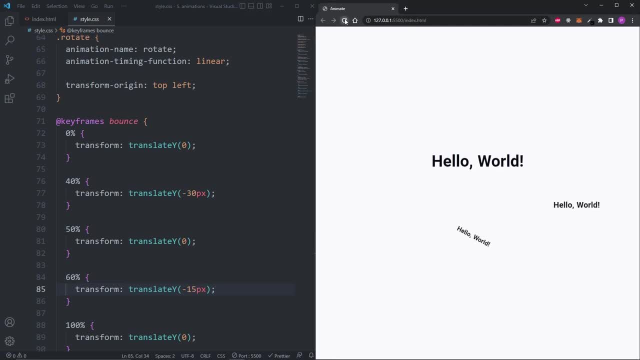 This looks pretty good, but we can still make it look better. Currently we're going from a translate y of 0 minus 30 pixels from 0% to 40%. To make it look snappier, I'll add a 20% with a transform. 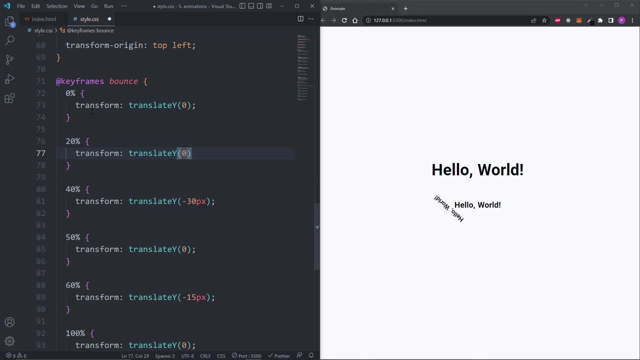 of translateY set to 0.. Now what's happening is from 0% to 20%. we're staying at 0. But now, starting at 20%, we can accelerate towards the minus 30 pixels and this will make our animation look better. It's subtle, but still better. We can do the same in between the 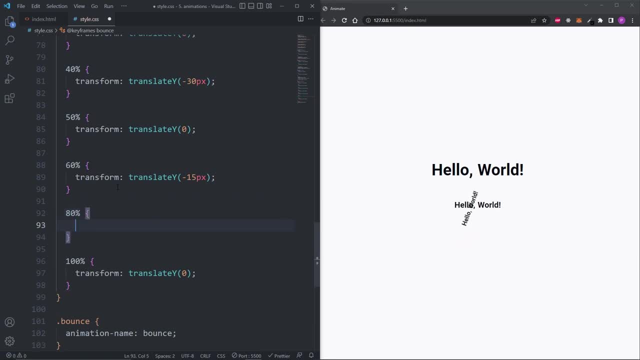 60% and the 100%. I'll add a 80% with a transform of translateY set to 0.. Our heading definitely looks like it's bouncing and the animation is exactly like I want it. However, inside our keyframe we are repeating ourselves a bunch of times with all of those translateY. 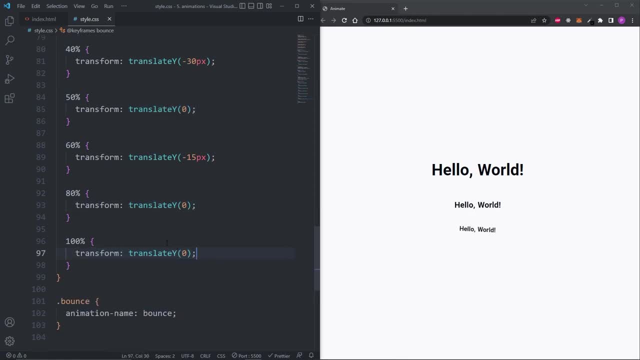 set to 0. In programming you really want to avoid repeating yourself. so to clean things up, all I have to do is remove all of the percentages where I'm repeating the translateY of 0. And then on my 0%, I can comma separate all of the percentages that had the translateY. 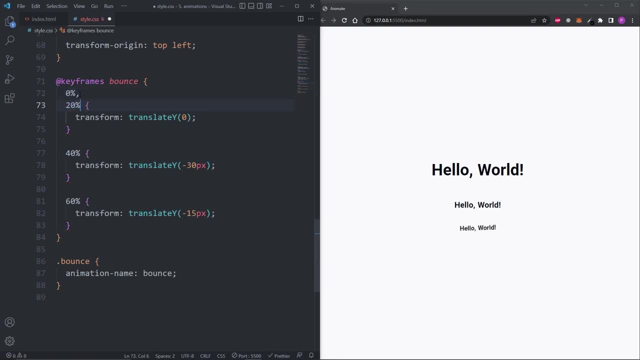 of 0.. So 0%, 20%, 50%, 80% and 100%. The reason this works is because keyframe percentages don't have to be in order. I could have the 60% be on top of everything and the animation. 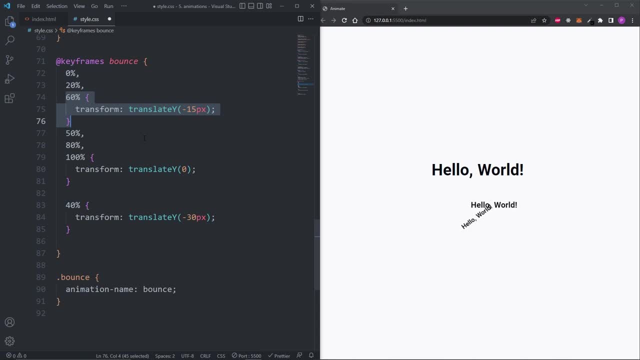 would still work perfectly. I'll bring it back down, though, just because I think it's cleaner and more readable. And there you have it. This is pretty much everything you need to know to start getting creative and building some beautiful animations yourself. If you enjoyed the video, I'd be. 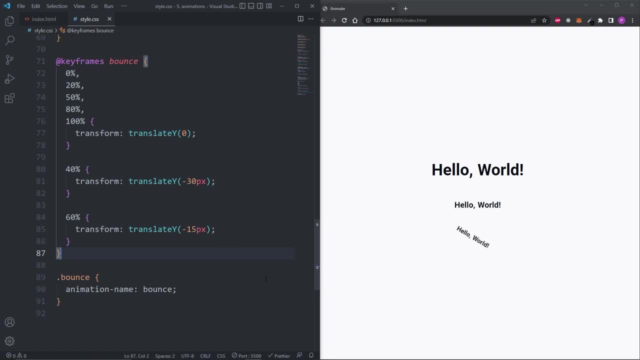 honored if you liked and subscribed. Thanks for watching and have a wonderful day. or even month to month like weather does. Climate is the average temperature and conditions in a place over a long period of time. The climate in one place on Earth is different than another place. For example, the climate in a desert can be hot and dry, while the climate in a rainforest is usually warm and humid. The climate in a desert can be hot and dry, while the climate in a mountain is usually humid. And in some mountain areas, the climate is cold all year long.